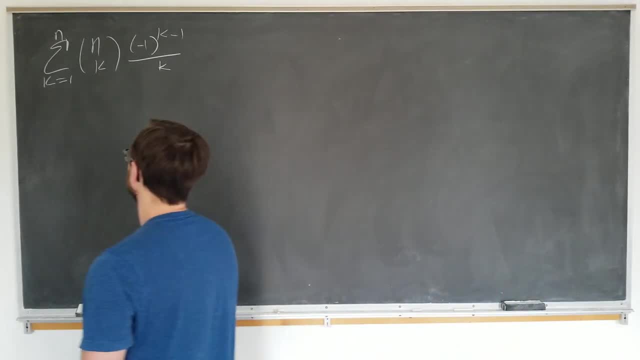 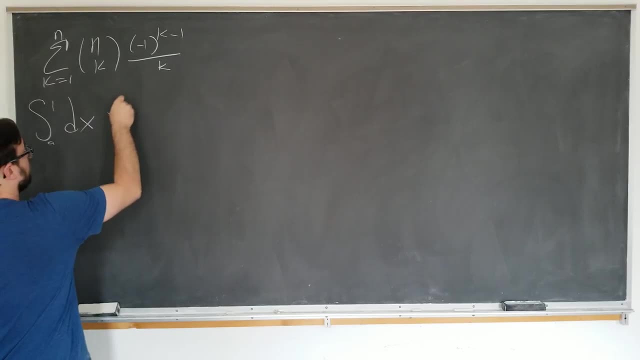 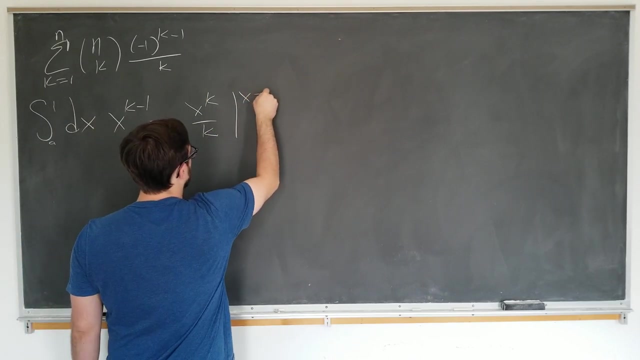 in order to get to the solution. So let's begin. First trick we're going to use is the fact that the integral from 0 to 1, respect to some variable x of x to the k-molecule, 1 minus 1 is equal to x to the k over k evaluated at x equals 1 and x equals 0.. 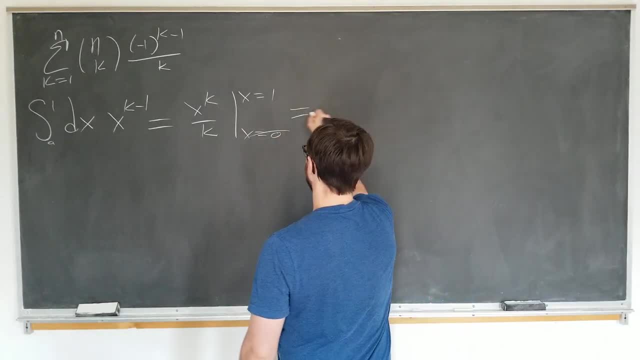 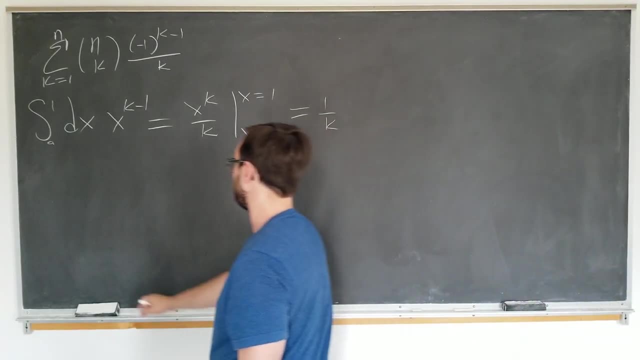 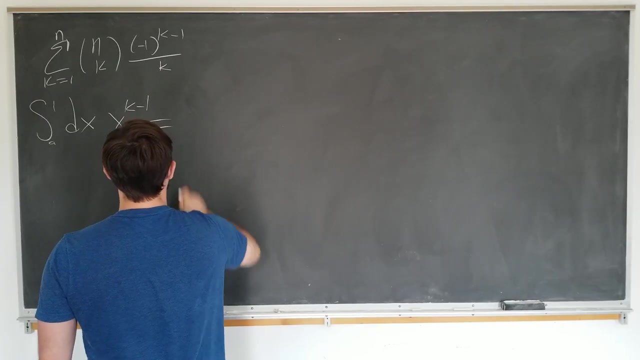 This limit becomes 0, of course. So the result is simply 1 over k, from x being evaluated at, x equals 1, of course. This is the first trick here. This is 1 over k. We're going to use this as follows. We see that there is no integral in the sum. 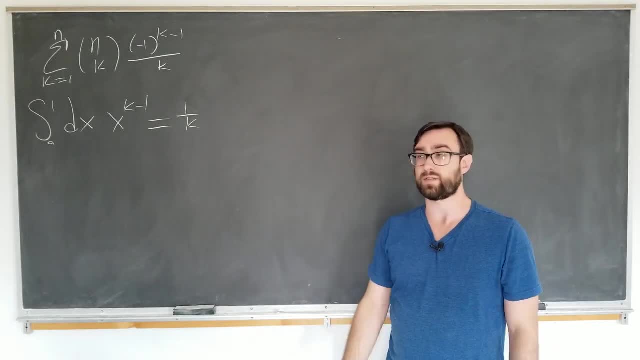 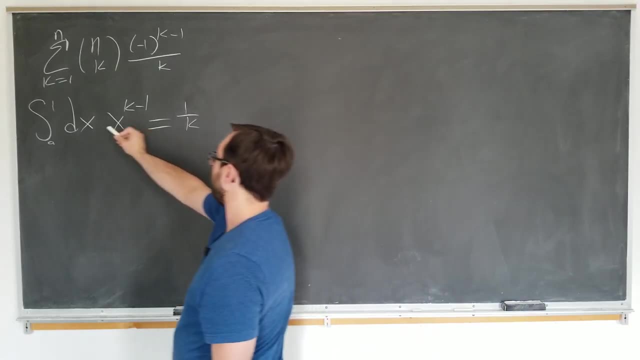 above. This is the only integral in the sum below of in the sum of. so we're going to use the integral above to interchange the limits of which is a standard technique in evaluating sums. We're actually going to introduce an integral with a new variable x that we can. 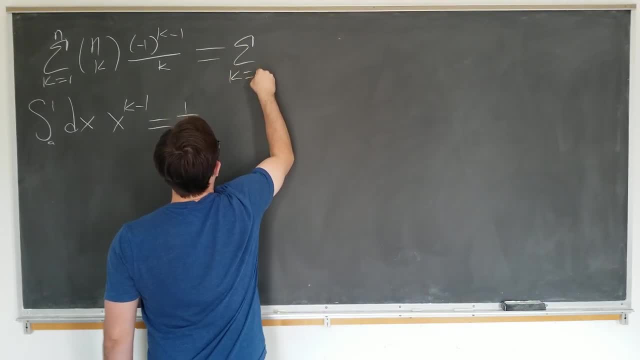 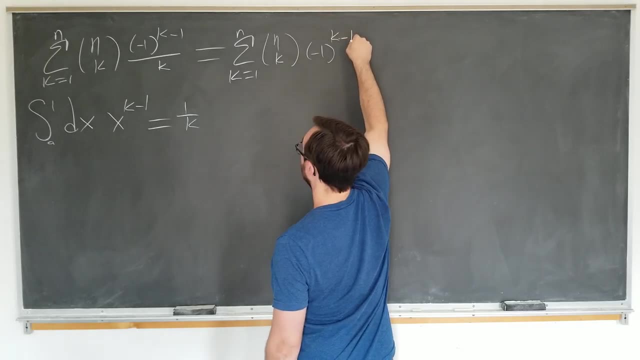 then interchange the limit of. so let's go ahead and write this now: Sum as k goes from 1 to n and choose k minus 1 to the k minus 1 power. Now we're just using a formula: 1 over k is equal to what we just derived from a. 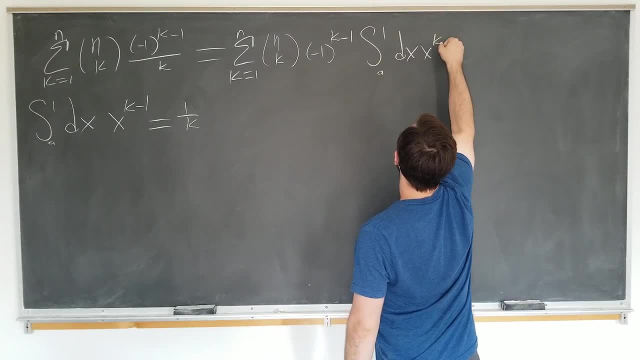 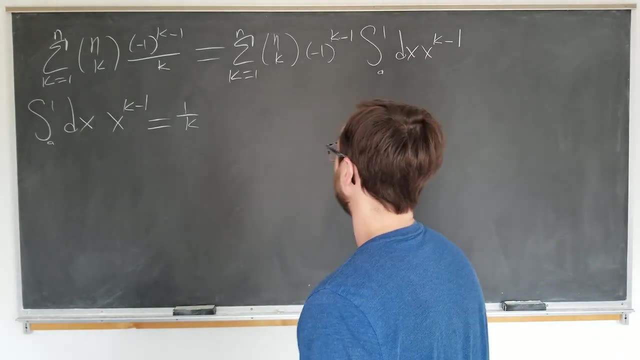 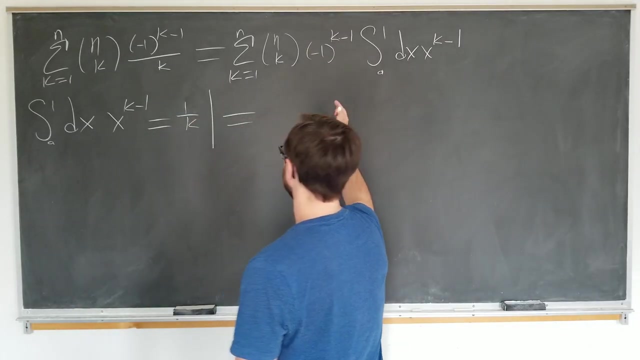 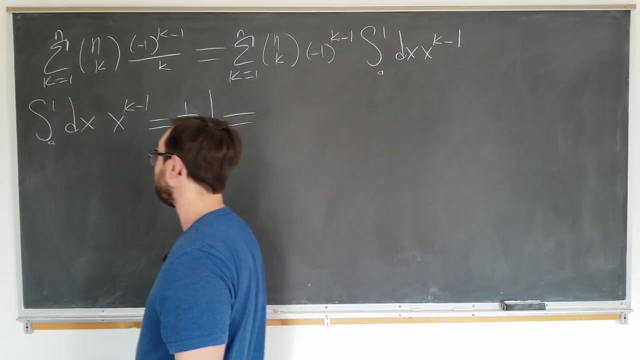 to the integral. and now what we want to do is interchange the order of the limits and write it as follows. so we want to interchange them now and we also want to take out a minus sign for what we're going to use in a moment, which brings us to the second trick. we are going to use the fact that minus 1 to 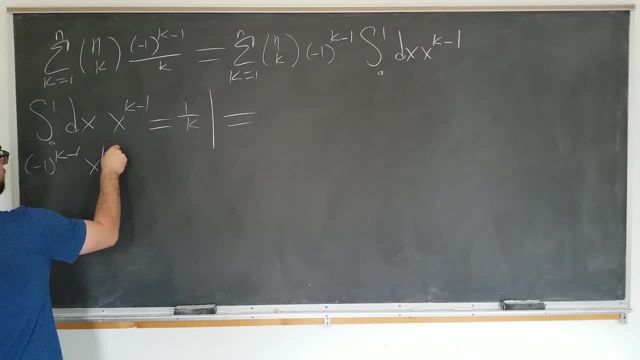 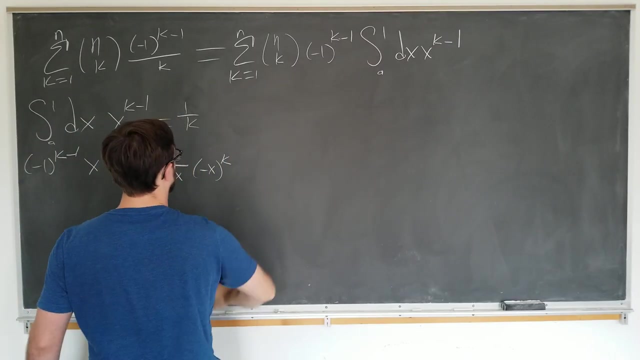 the k minus 1. x to the k minus 1. we're going to use in the following form: it's going to be written here as minus 1 to the x, minus x to the k, for reasons which will become clear soon, and we write our sum in the following format: it's going: 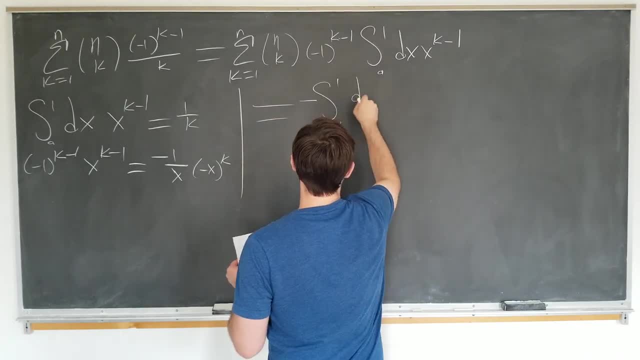 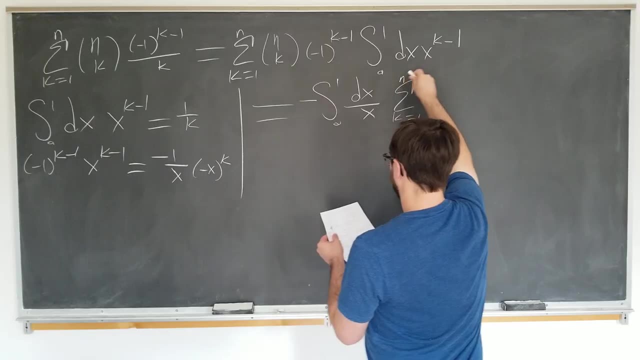 to be minus the integral from 0 to 1. it's back to our new variable, X divided by X. Now we have the sum on the inside as k goes from 1 to n. we have binomial coefficients, n. choose k of minus x to the k. 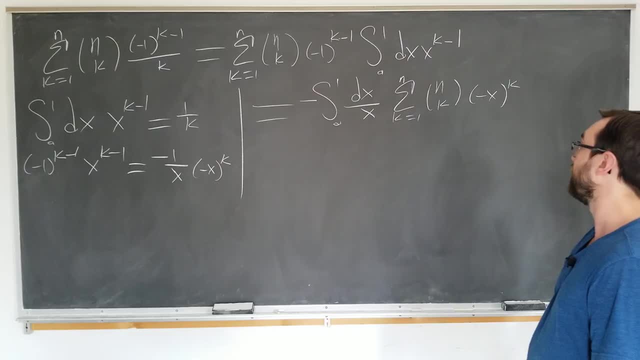 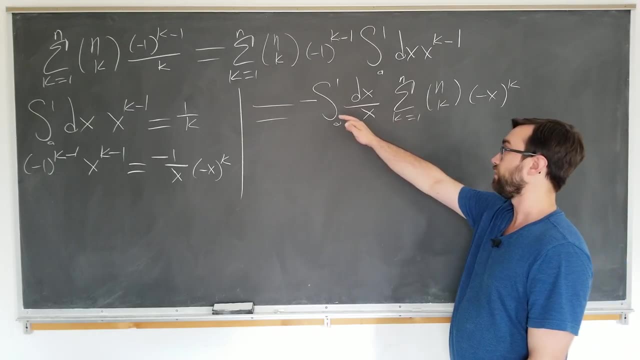 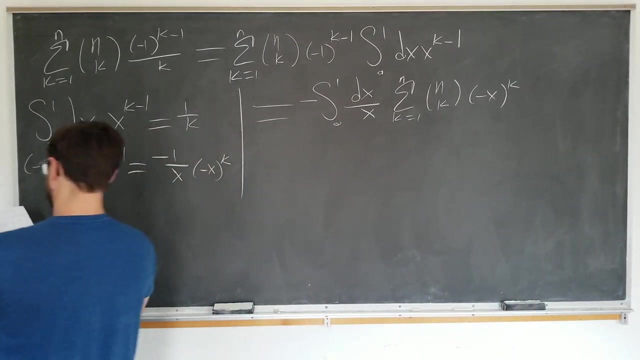 So basically we have a sum here that looks something like a binomial series, which we should know how to evaluate. So we're stripping away the alternating behavior so we can get to the binomial series, Which brings us to our third trick. We're going to note that the sum, as k goes from 1 to n- n choose k minus x to the k is: 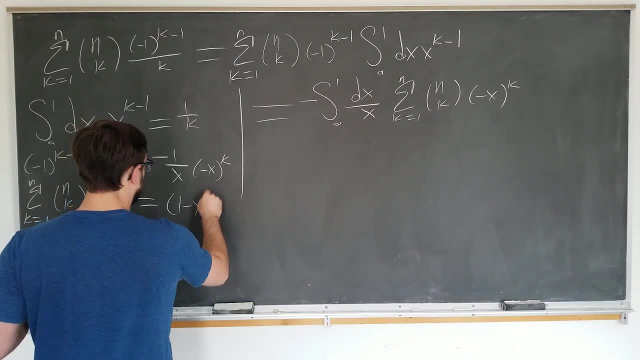 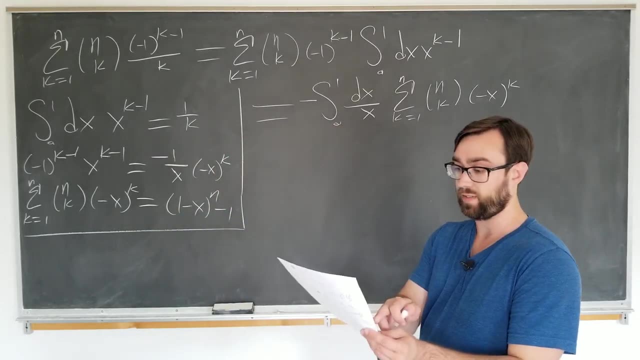 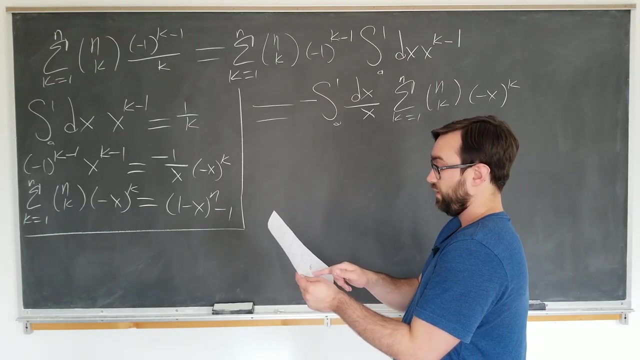 actually equal to 1 minus x, to the nth power minus 1.. Why is this true? Well, it's pretty straight forward, actually, Make sure I got it right here first. See, I just have to use my notes. There are just so many tricks in this video. I can't do it without my notes. 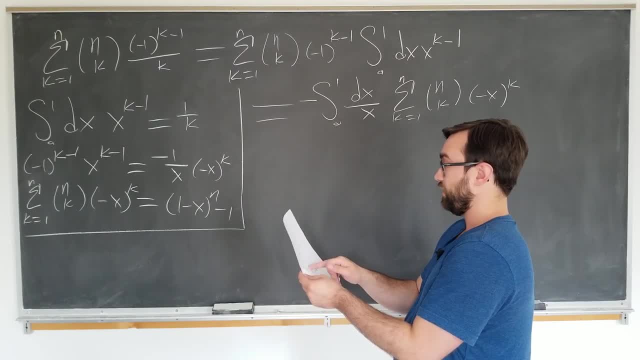 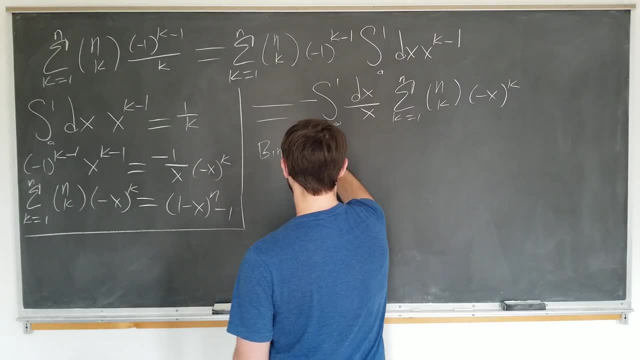 Yeah, so sum k goes on from n- n. choose k minus x to the k. Exactly okay. This is true because the binomial theorem, or binomial expansion as we call it in physics, states that if we have a quantity 1 plus x to the n, n is typically taken to be small. 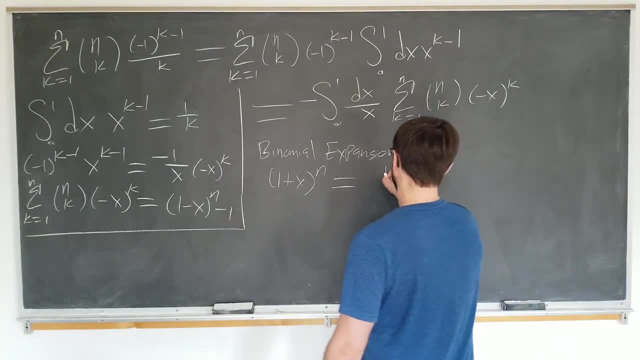 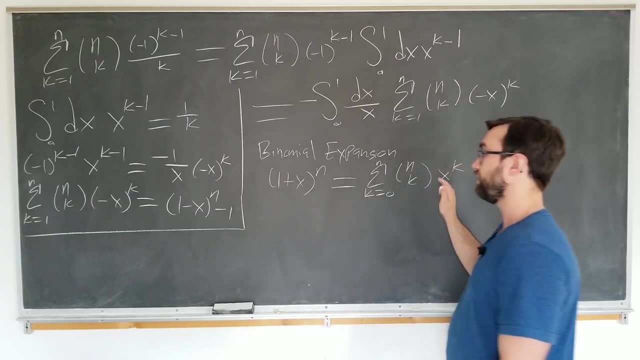 in physics, but we're doing math here. So x is 1 plus x to the nth, power minus 1.. x is arbitrary, is the sum as k goes from 0 to n of n. choose k, x to the k. This is not quite what we want. 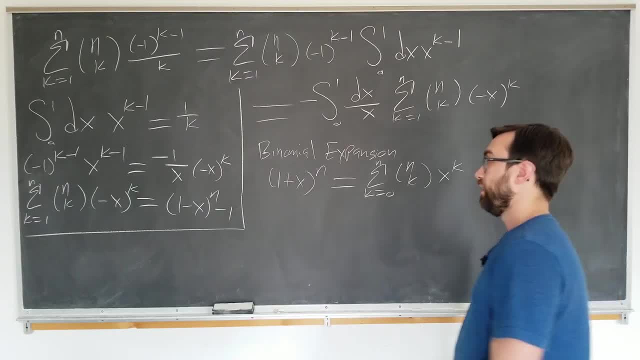 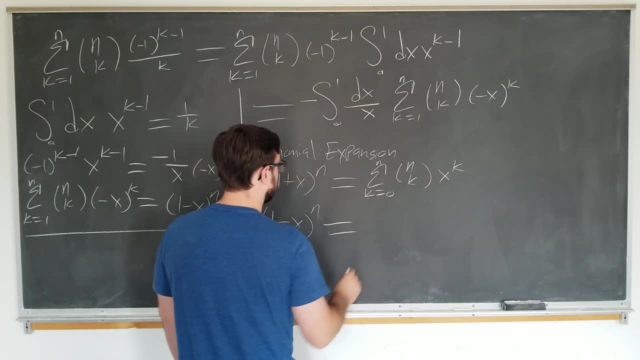 We have the index starting at 0 instead of 1 here, and we have an x instead of a minus x, so we can fix that. So 1 minus x to the n is now equal to. we're letting x go to minus x in the expression. 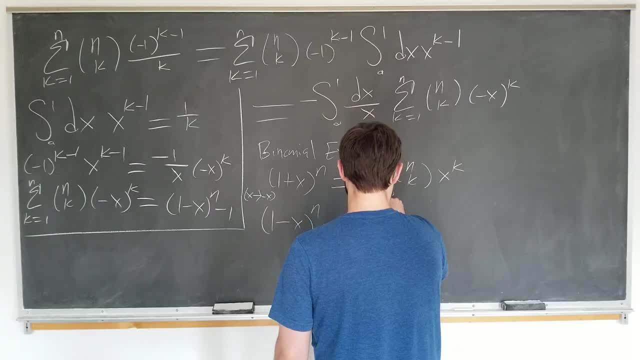 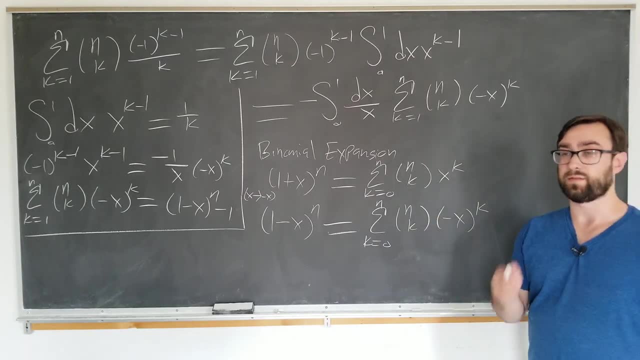 here. So it's k equals 0 to n. n choose k minus x to the k and finally we're going to write out the first term of here. So the k equals 0 term is simply 1, and then we have what we want, as k goes from 1 to n. 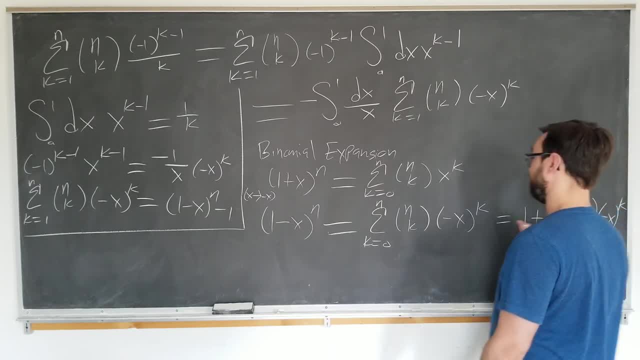 and choose k minus x to the k, and then you simply subtract 1 on both sides and you get the result that you seek here. It's pretty much a trick- yeah, lots of tricks here- but this is how you do it: Subtract 1.. 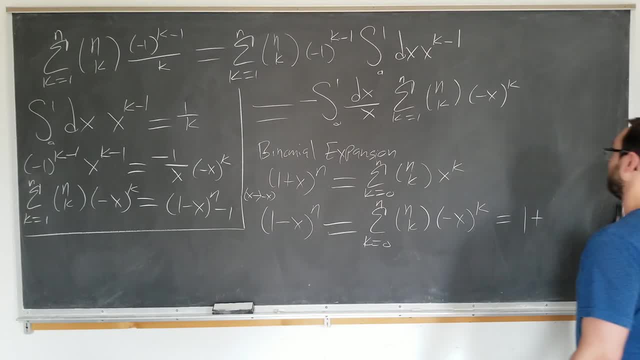 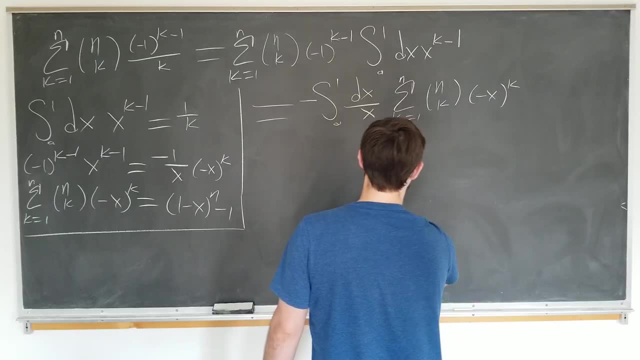 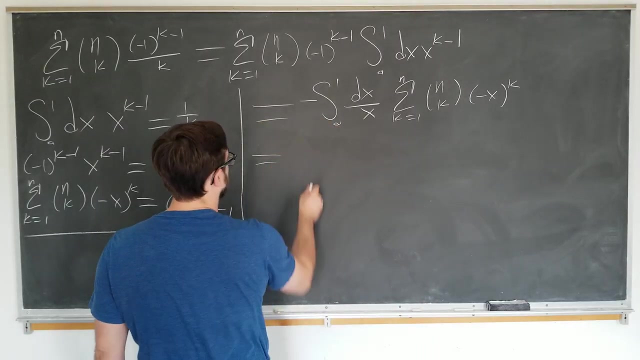 Subtract 1 over there. get what you want, Excellent. There is one more trick. we'll get to in a moment. First, we're going to write down what we just derived here. We're going to note that this is now minus integral from 0 to 1 dx over x. 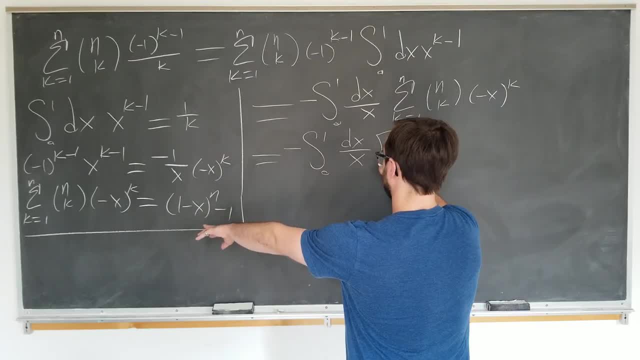 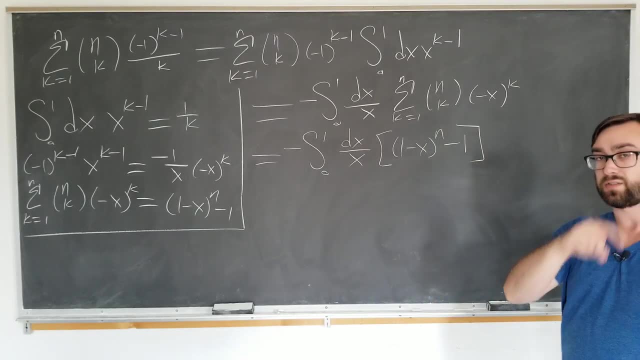 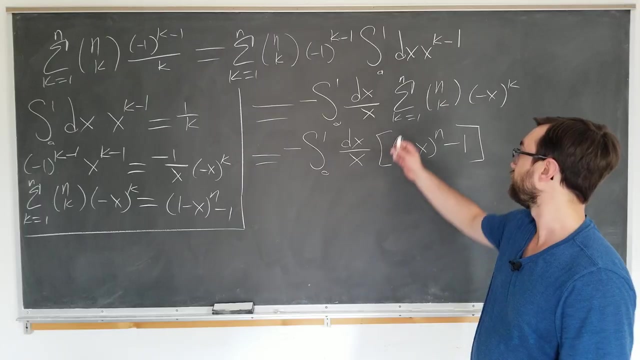 We're just going to put the sum here. This is actually equal to 1 minus x, to the n Minus 1.. So you see what we've done here. We interchanged the values, sorry, the order of operations. We did the integral second. 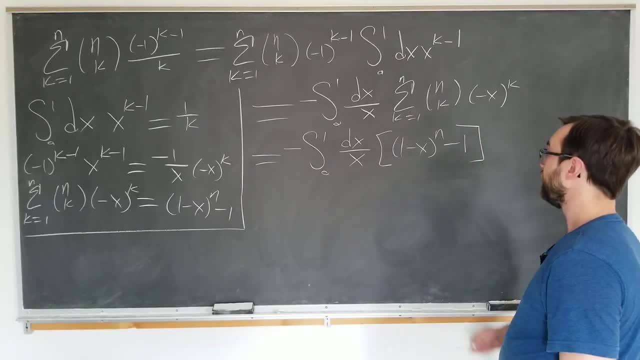 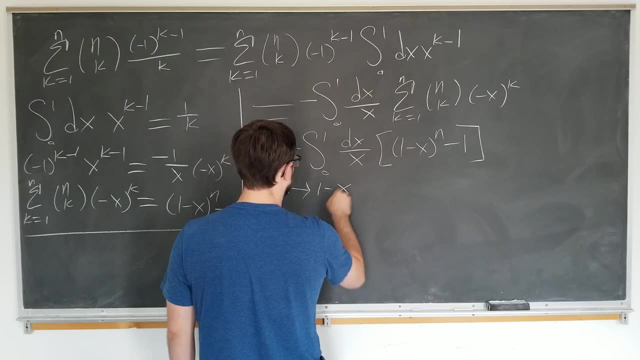 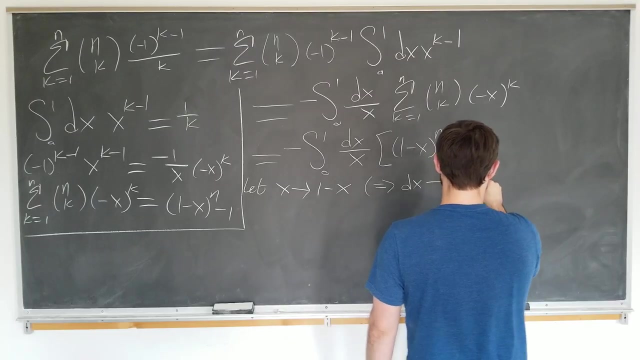 We did the sum first and now we're going to do the integral. since it's easier to do that, Let us now make a substitution. Let x go to 1 minus x, which of course tells us that dx goes to minus dx, And we also have that 1 minus x goes to 1 minus 1 minus x, which is actually equal to. 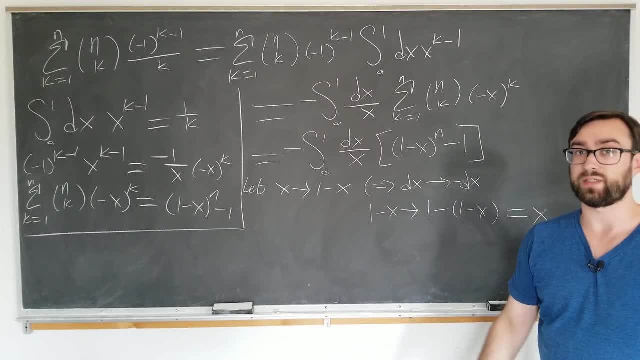 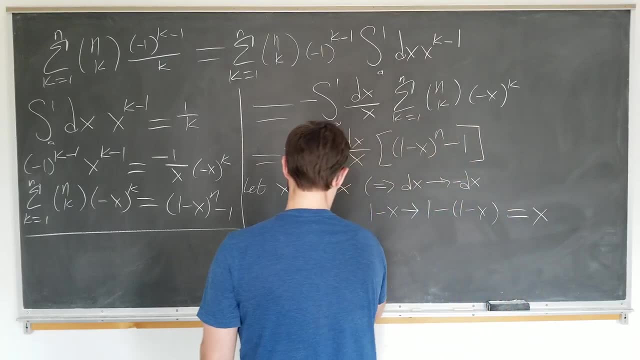 x. This is an important function of the property. sorry, important property of the function. 1 minus x is actually self-evolutional. It satisfies the differential equation. f of f of x is equal to x. It's not an idempotent. 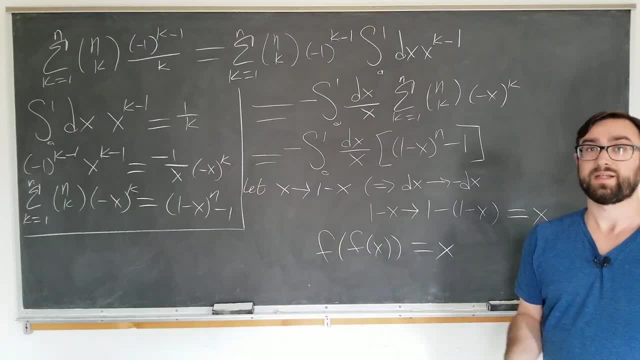 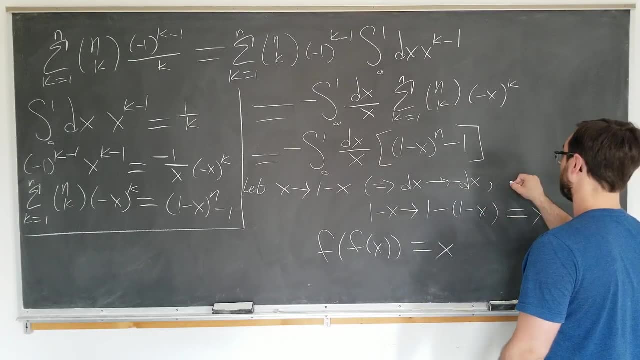 But you know, It's not an idempotent, It's an integral. It satisfies this. I forgot what it's called. Let's move on, Okay. So 1 minus x goes to x And of course we have x itself goes from 1 to 0.. 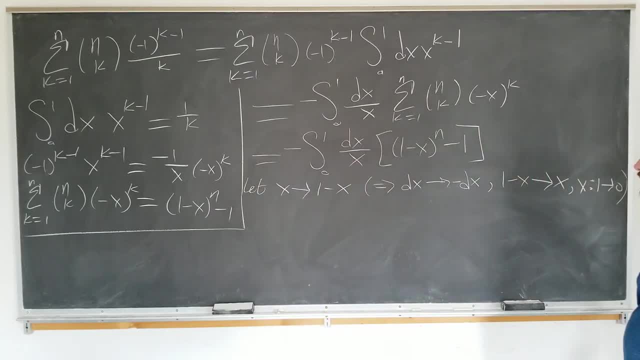 Excellent, Now we can transform our integral. We're just going to replace all instances of x by 1 minus x, All instances of 1 minus x, All instances of 1 minus x by x. We're going to put the minus sign for the dx and we're going to interchange the limits. 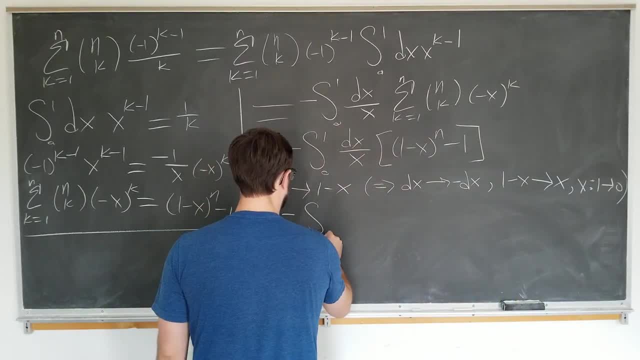 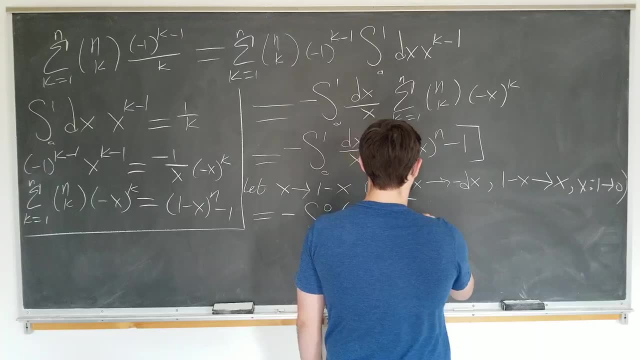 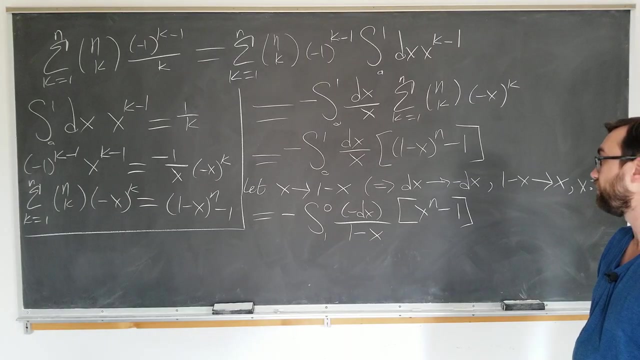 of the integral Minus integral, from 1 to 0, now Minus dx. over 1 minus x. Now we have x to the n minus 1.. We are going to now note that these two minus signs cancel And Excuse me. 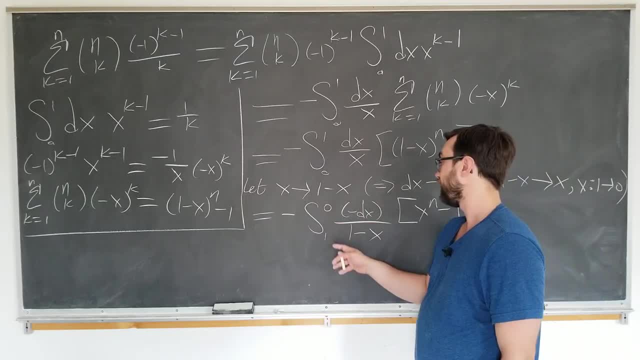 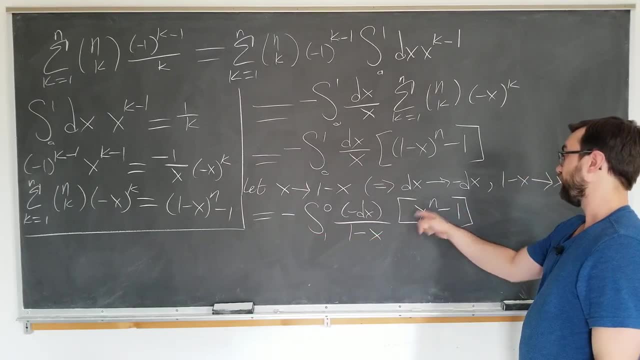 We want our integrals to go from 0 to 1.. So we're going to introduce another minus sign outside And we're going to put it into this factor here. So we're going to reverse the order of these factors, So our final result becomes integral from 0 to 1 with respect to x of 1 minus x to the. 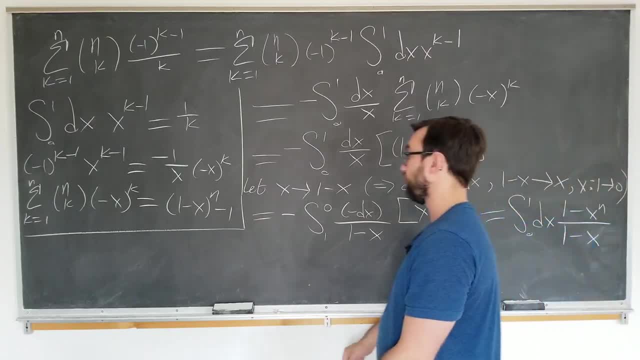 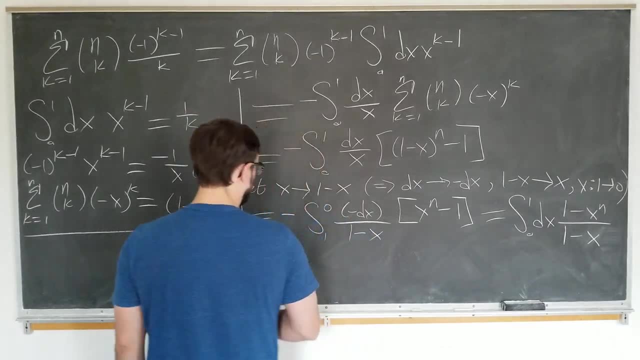 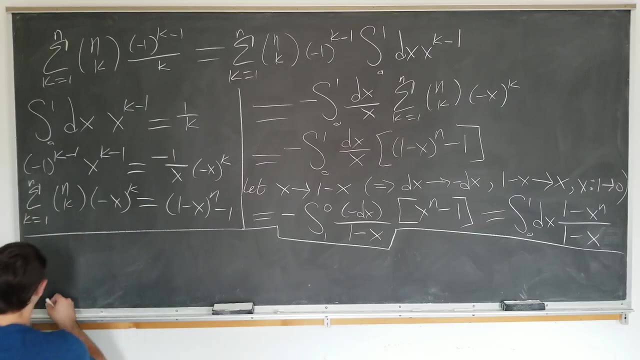 n over 1 minus x, Which to most viewers- hopefully you should recognize the integrand as being nothing but a finite geometric series which we can readily integrate as follows: Integrating now, Our result is the integral from 0 to 1 with respect to x, of 1 plus x plus x squared plus. 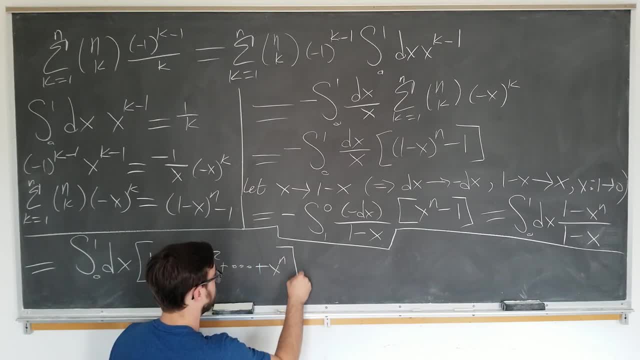 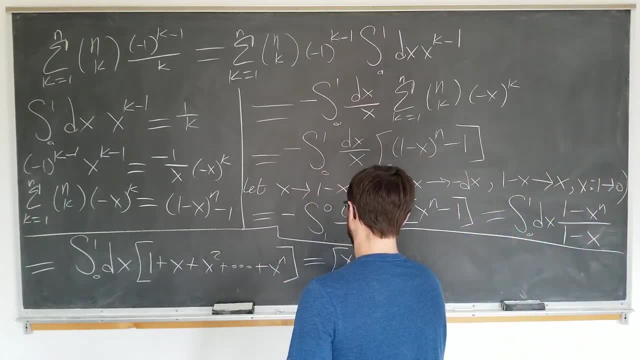 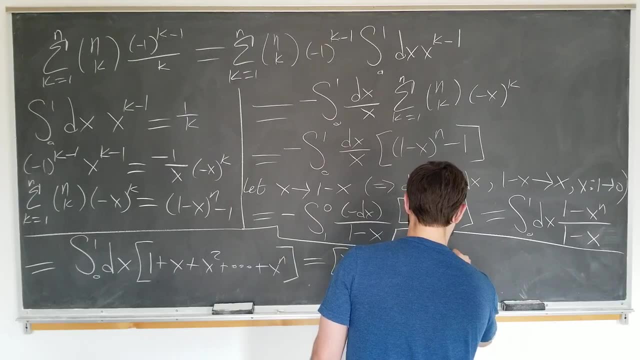 Of course, Of course, Of course. It's just simply x plus 1 half x squared plus 1 cubed. Sorry, 1 third x cubed plus higher order terms Till we get to 1 over n. x to the n. 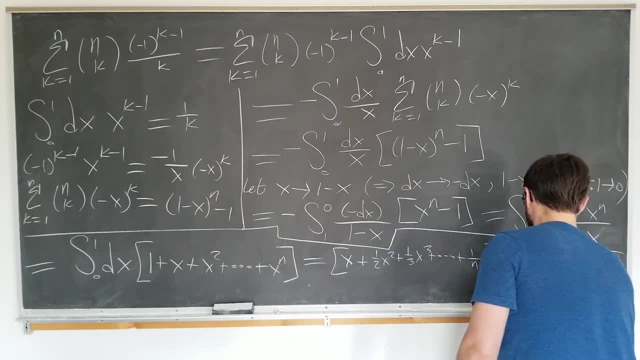 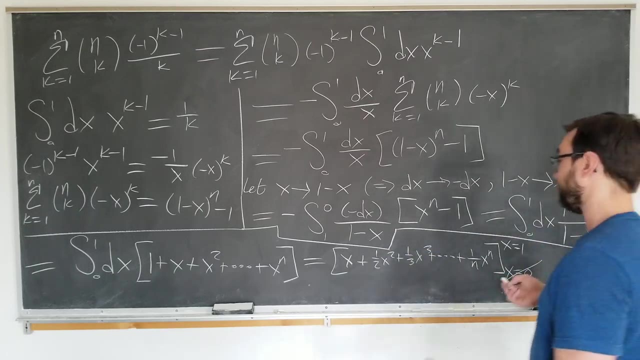 Evaluated at: x equals 1, x equals 0.. Again, we see that the lower limit cancels out. That's just looks bad. Lower limit cancels out Since there's a power of x everywhere, so we have to evaluate this. x equals one, so it's just. 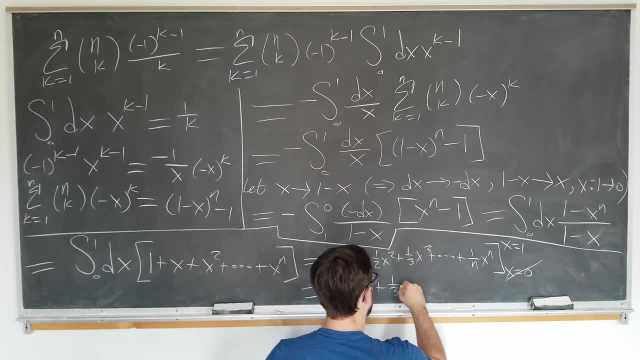 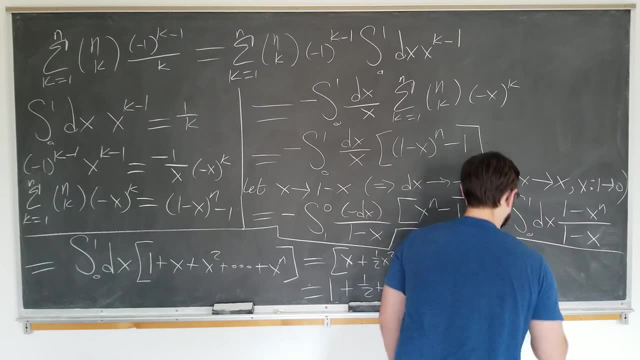 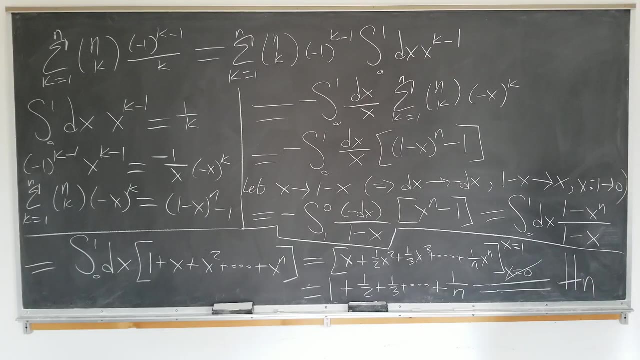 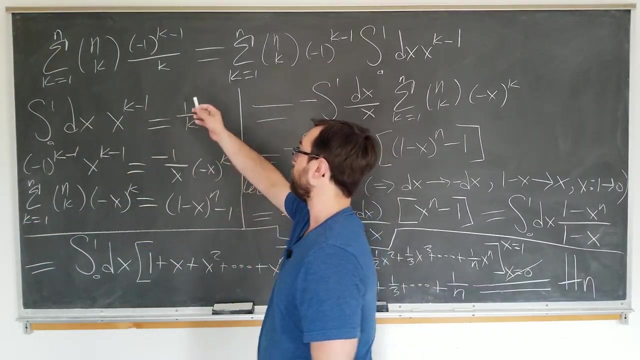 one plus one half, plus one third, plus higher terms, all the way to one over n, which many viewers could recognize, recognize as the nth harmonic number, h, n. so this is actually a pretty surprising result. we have the alternating series of binomial coefficients with a weight of one over k, inverse weight. 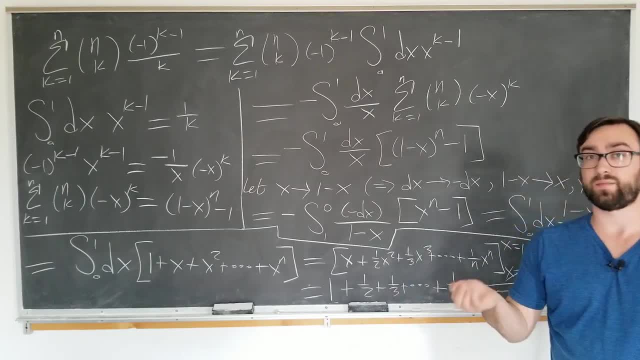 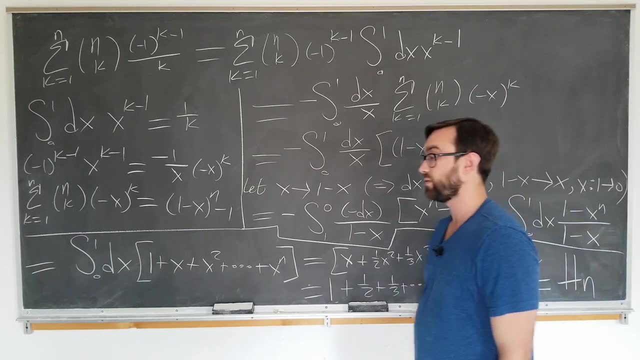 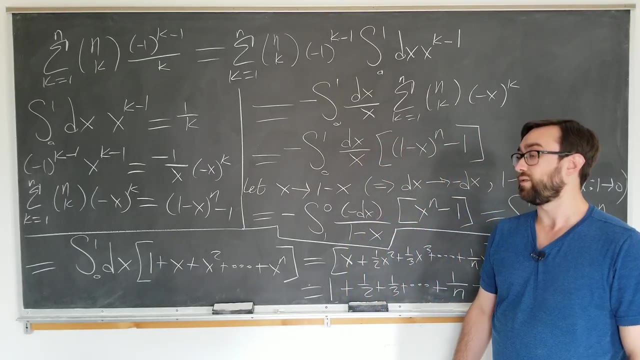 actually removes all of the alternating behavior, resulting in a sum of the reciprocals of the integers themselves, and that's pretty much the main result of the video today. you might ask yourself: why did i do this? what is the utility of this formula? well, the main reason, like i indicated, is some indian kid challenged another. 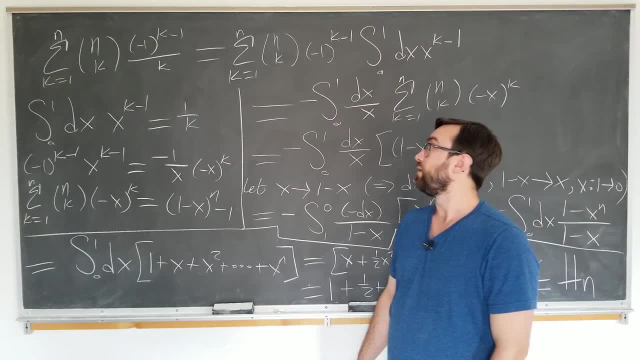 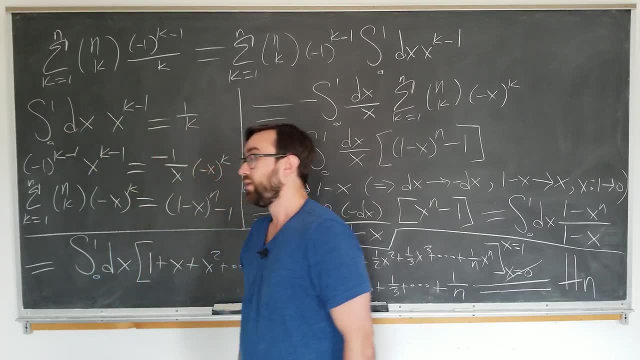 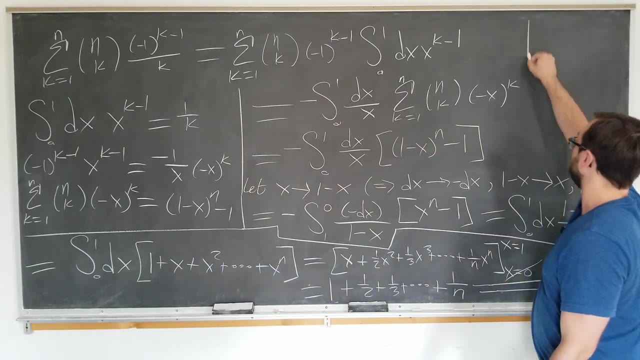 indian kid. so if an indian kid challenges you on how to evaluate a sum like this, you might want to use the first trick here: introduce an integral so you can interchange the limits. there are other reasons as well. if you are good enough, i'm i'm actually not good enough to do this. i don't quite understand. 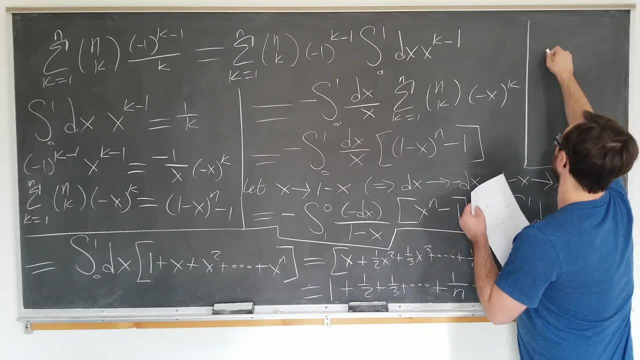 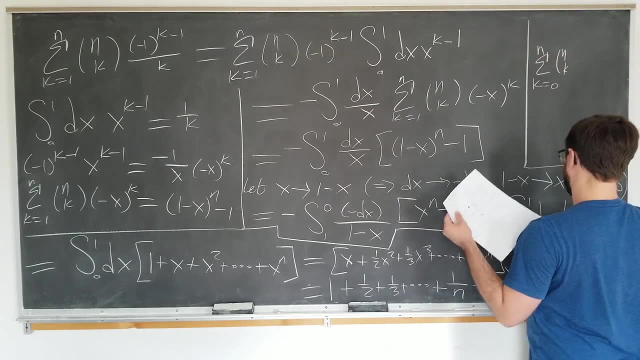 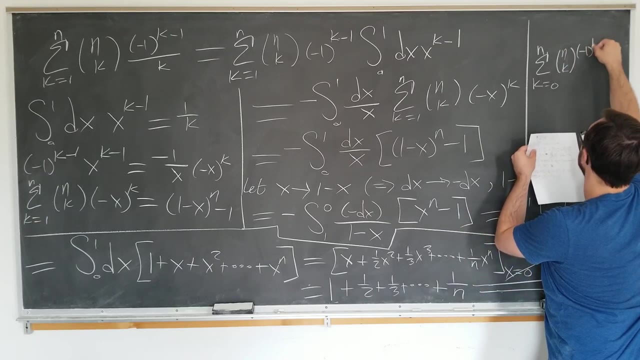 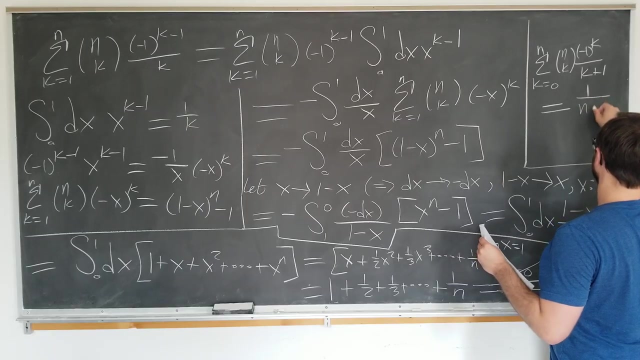 how this is done, but i know it's possible. if you wanted to, you could also use this result to evaluate this: sum k equals zero from n and choose k minus 1 to the k over k plus 1.. you can show that this is actually equal to 1 over n plus 1. 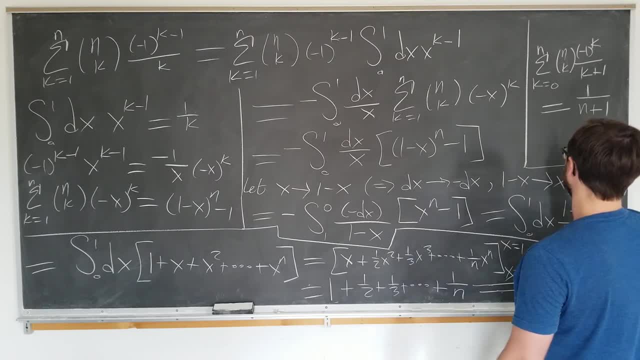 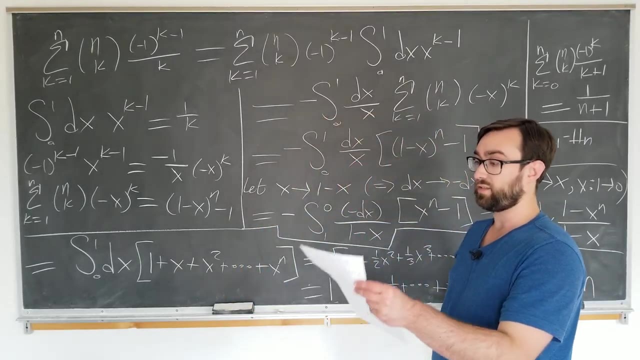 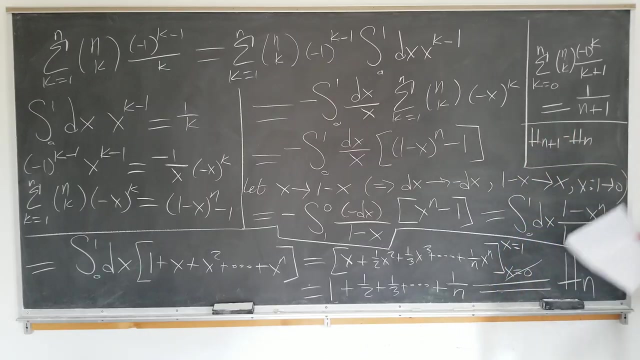 which you can imagine. the final result is subtracting h n plus 1 minus h n, which of course is 1 over n plus 1. over m plus one, since all the intermediate terms cancel. there's just a lot of tedious index manipulation which i don't quite fully understand, so i can't include it in this video. but this is: 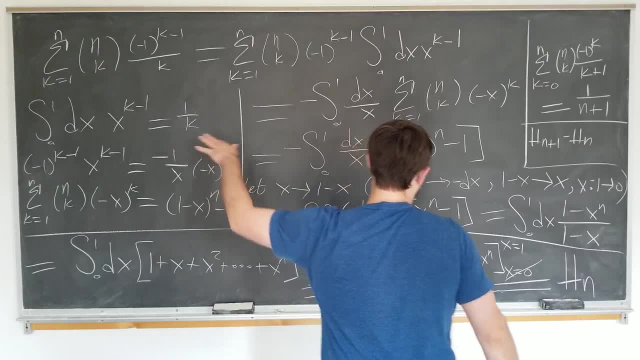 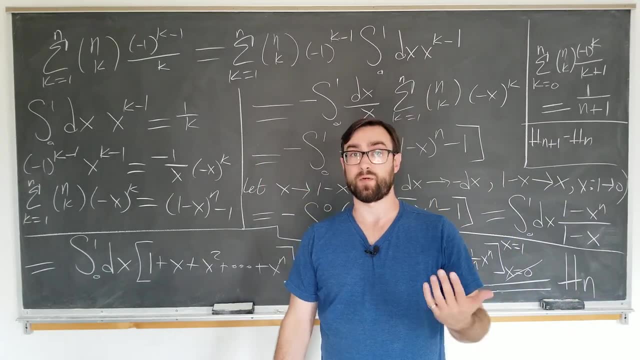 one use of this binomial series. if you wanted to evaluate a different binomial series, you wouldn't necessarily have to go back to the integral switching, though of course you could if you wanted to and if you enjoyed this one. to see more math, please subscribe to my channel. i'll see you.